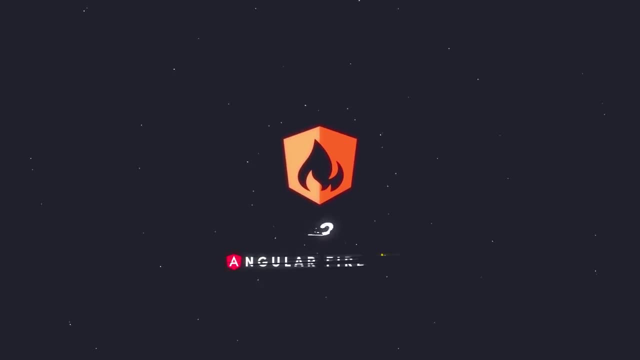 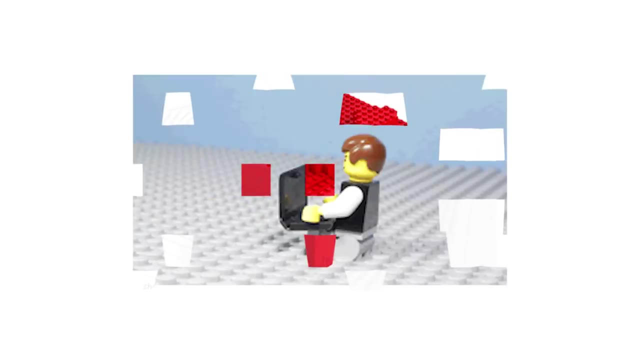 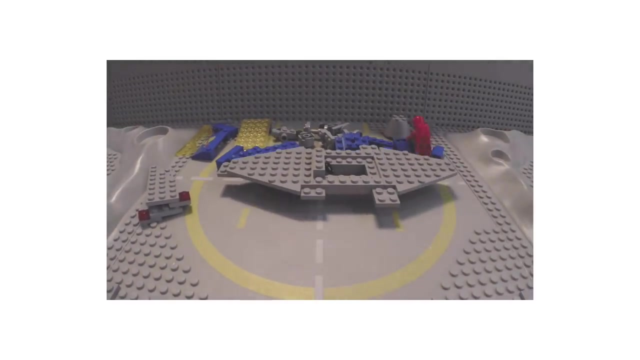 Components are like the Lego pieces of an Angular application. If you don't know how to put them together properly, you're not going to be able to build anything cool. Over the next 10 minutes or so, I'll show you all of the basics in Angular components and how to piece them together in an 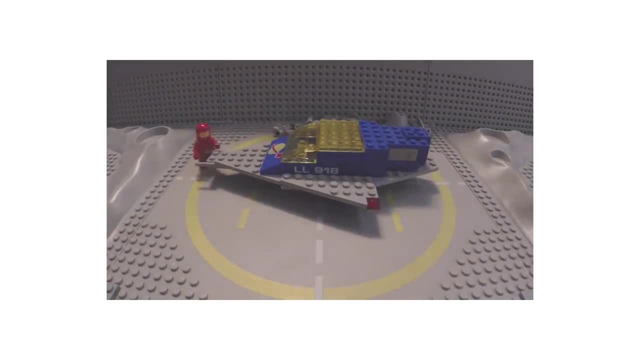 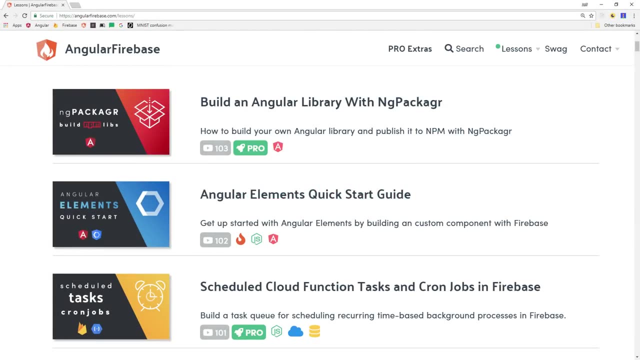 application. This video is beginner level, so if you know a little bit about JavaScript and web development, you should be okay. If you're new to the channel, make sure to like and subscribe and grab the full write-up from angularfirebasecom. The first question we need to answer is: what is a? 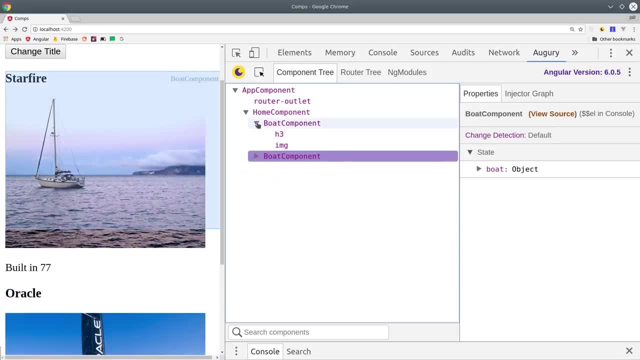 component in the first place? And I think the most simple answer to this question is that it's just a controller for the user interface. As a developer, you write components to control how your app is experienced by end users. To show you this in practice, I'm opening a brand new Angular 6 app. 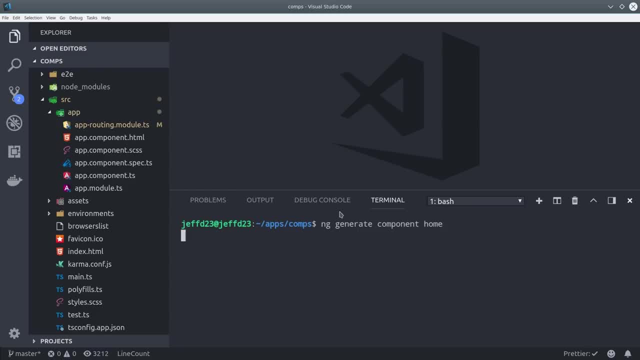 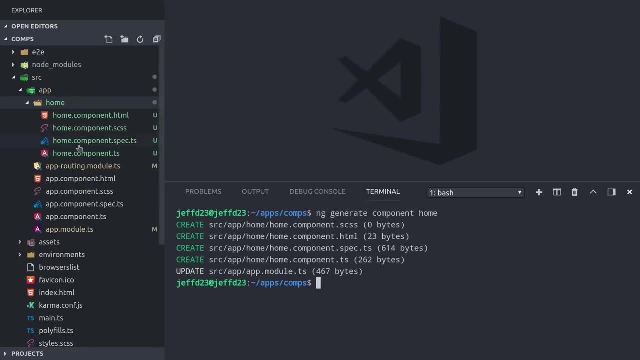 that was generated with the CLI. Then I'm generating a new component called home, which, you'll notice, creates four different files in the app directory. The vast majority of the logic that you'll write will be in the home-componentts file, The component: 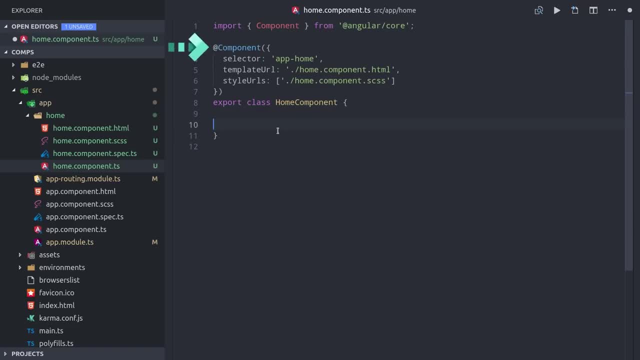 itself is just a TypeScript class, but it uses this component decorator to sprinkle in some Angular magic. The most important thing is that it allows us to bind data from this TypeScript file to the HTML template. The first thing I want to show you is how to bind TypeScript code to your HTML. 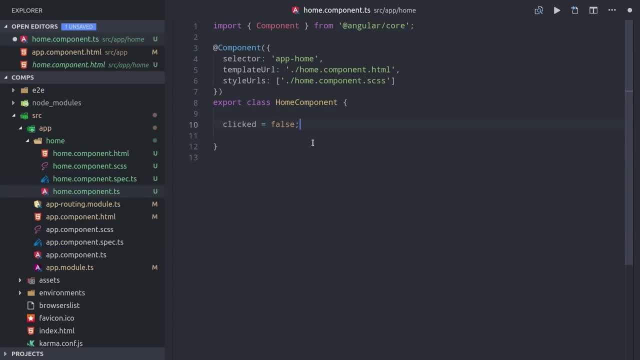 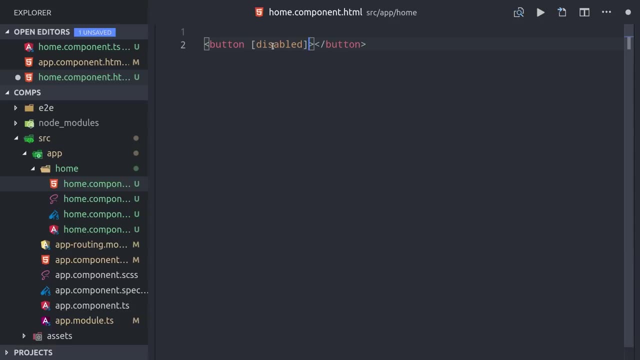 Let's define a property on this class called clicked, that defaults to false. Now let's go into the HTML and let's imagine we have a button that we want to disable after it's been clicked. We can bind our TypeScript data to this attribute in HTML by wrapping it in square brackets. 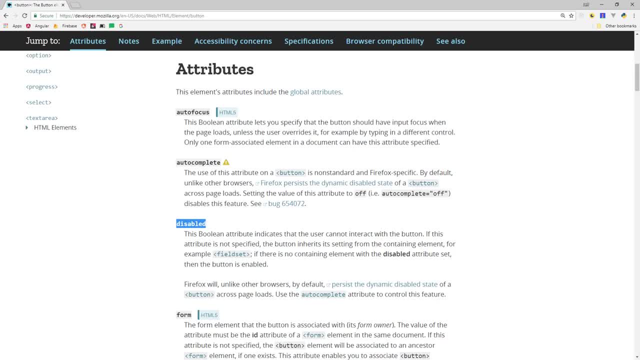 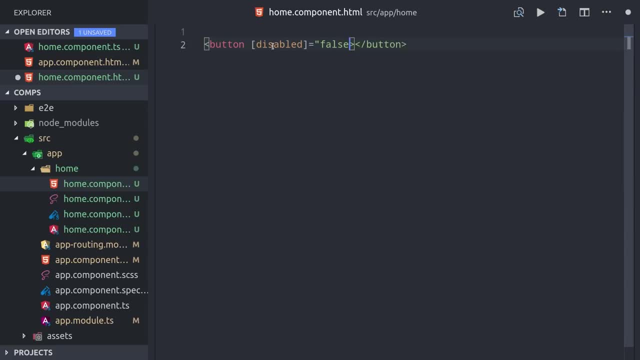 Disabled isn't something Angular provides. it's an actual attribute on the HTML element which I'm looking at here in the Mozilla documentation. The special thing about Angular is that we can wrap this attribute in square brackets and then bind it to our TypeScript, So instead of just passing it, 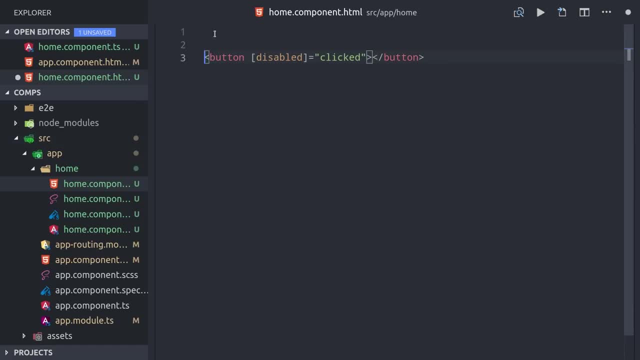 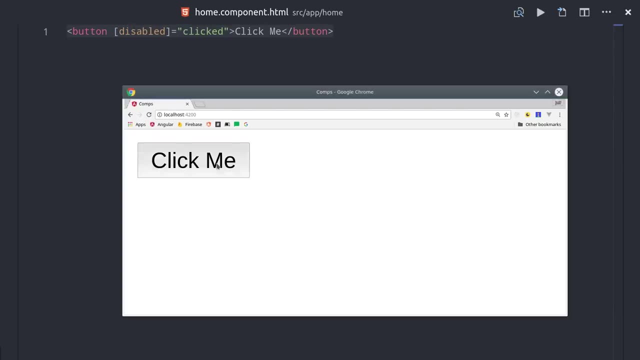 a boolean value like false, we can actually pass it our clicked property, which we can then toggle TypeScript as needed. It's currently set to false, so we should be able to serve our app and the button should be clickable, which it is, If we go into TypeScript and change our clicked 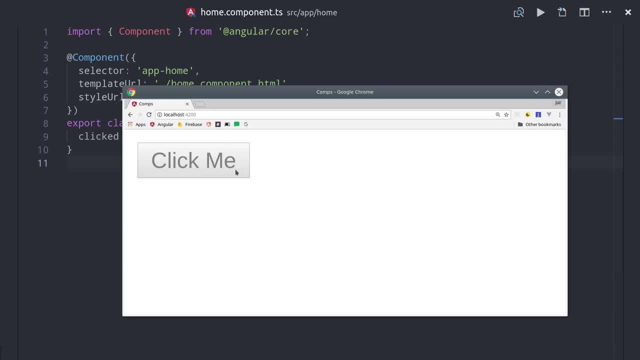 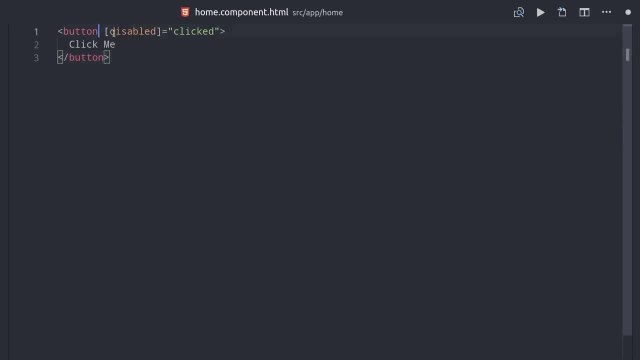 property to true, you'll see that the button is now disabled and unclickable. In addition to attributes, we can also bind to events that happen in the HTML. So let's say we want to change this button to disabled after it's been clicked once, We can use parentheses to bind to the click. 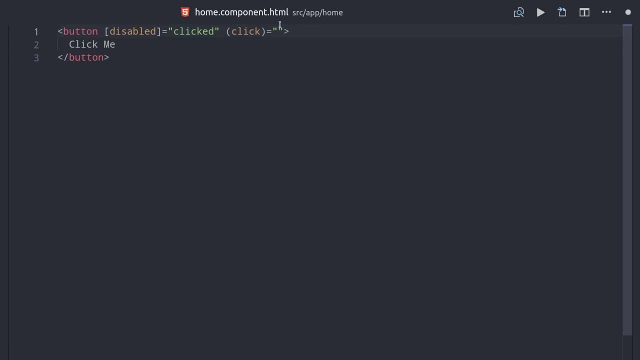 event on this button and then we'll pass it a function that will define in our TypeScript to handle this event. Now we can switch back to TypeScript and define this event handler method. We currently have the clicked property set to false, but we want to set that to true once. 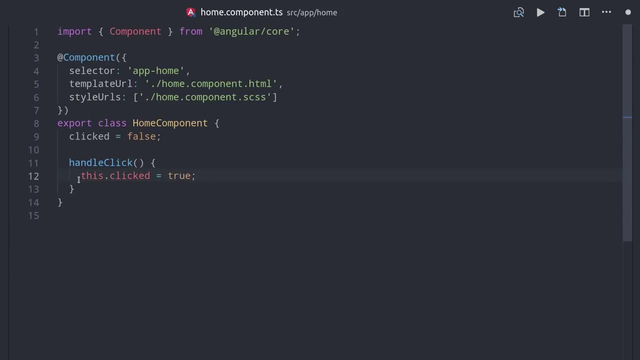 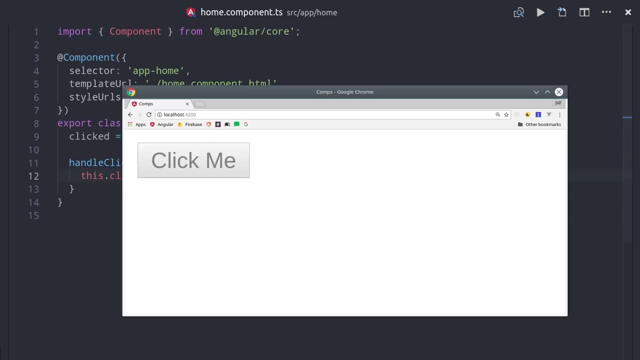 the button is clicked, which we can do by calling this clicked equals true. When we click the button, this handler will fire and then the button becomes disabled because it flips that property to true. That's how you bind to events and attributes in Angular. but one other fundamental thing. 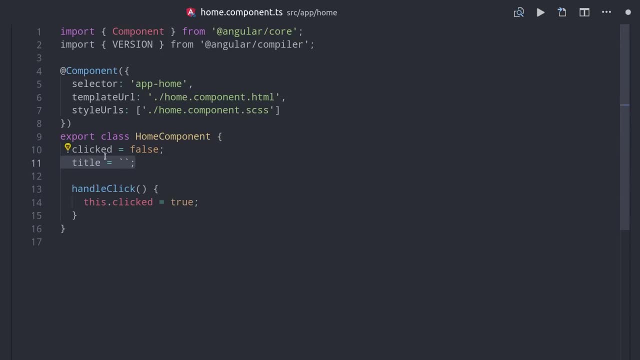 is interpolation And basically all that means is we're taking a raw value from our TypeScript and rendering it out in the HTML. So, for example, let's say we have the title here that shows the Angular version that we're currently running. So the title is just a string value that gets. 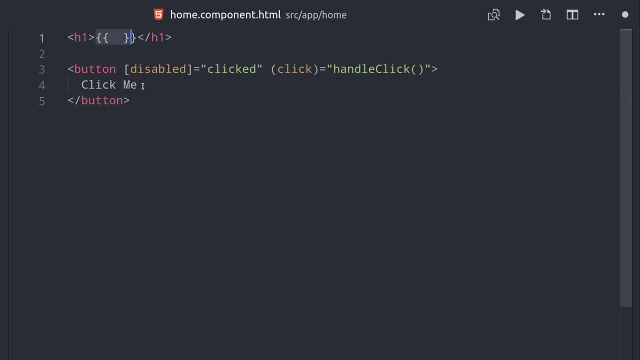 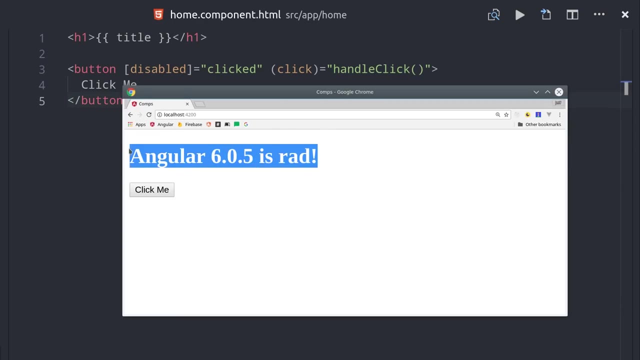 created dynamically, and then we can go into our HTML and use the handlebar syntax to interpolate it into the template. If we reload the browser, it should show us that we're running Angular 6 for this project. So now that we have a working component, how do we actually use it within the 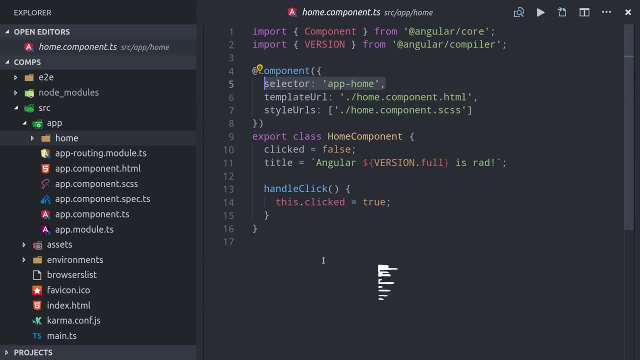 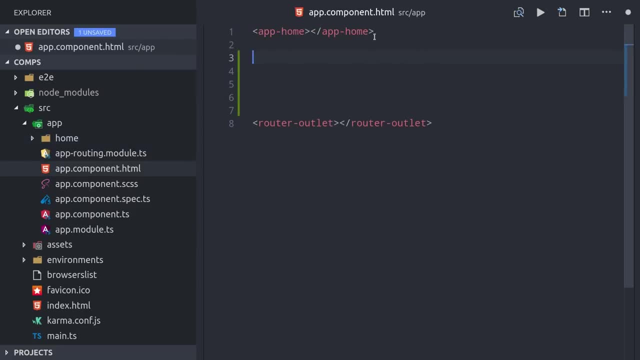 context of our Angular application. The most basic way is to declare it in the HTML with its select, which in this case is just app dash home. If we go into this project's app component, we can just declare our app home page there, and it will be rendered out like it's just a regular. 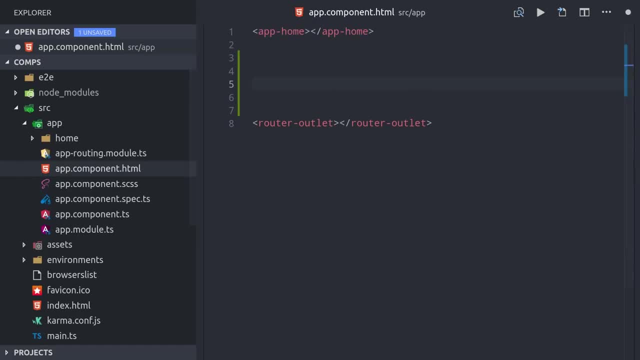 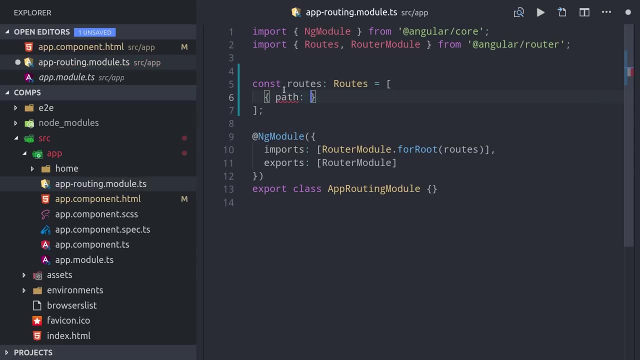 HTML element, But we can also load it with the router and have it appear where this router outlet is based on a certain URL path. Check out episode 113 to learn all about the router. but the most basic use case is that we set up a path and then we point this path to our component. 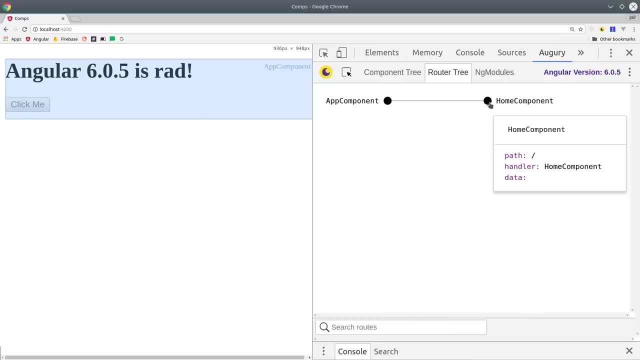 If we reload the app in the browser, you'll see it looks exactly the same. but if we open up the Augury plugin and go to the router tree, you can see that it's being loaded by the router instead of just the HTML directly. You can also load components dynamically. 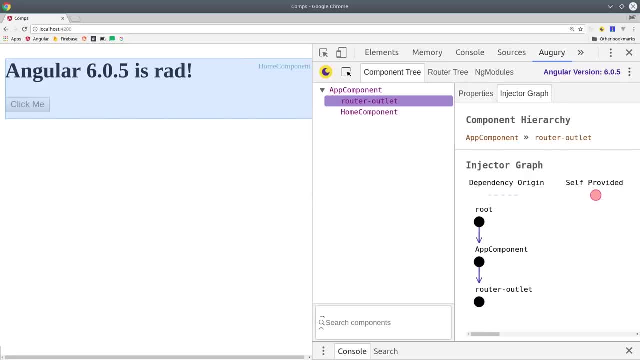 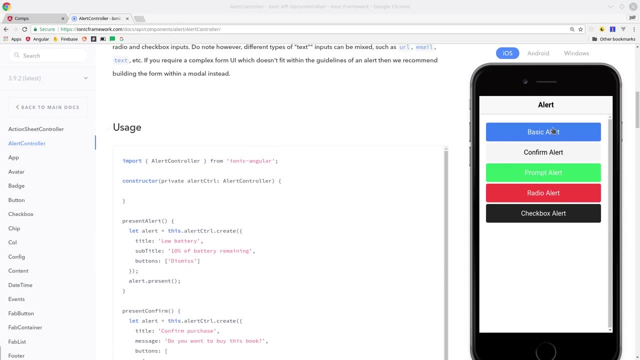 but without changing the route. A common use case would be like a popup or modal window. This technique is used frequently in the Ionic framework. For example, the alerts controller will dynamically load an entry component whenever the button is clicked. And lastly, the cool new way to load a component is with Angular Elements. 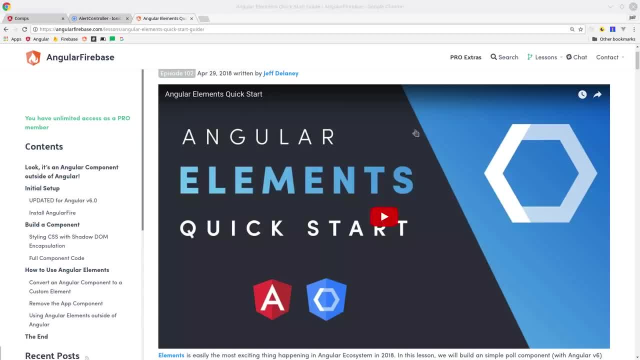 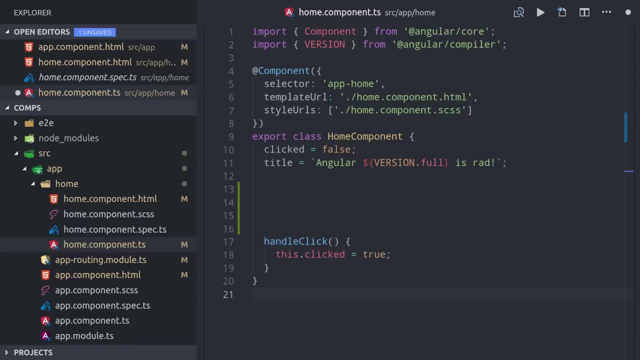 which allows you to convert it to a regular web component and then use it outside of Angular completely, So you could just drop it into a regular HTML page, which you can learn all about in episode 102.. The next thing we're going to look at are directives, and a directive is basically: 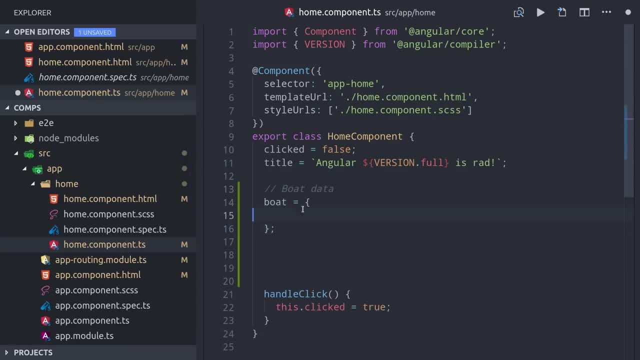 just like a component, but without its own HTML or CSS. Instead, it attaches to a host element and changes the behavior of it. To demonstrate this, I've added an object called boat with some dummy data to our component. Then perhaps the most useful built-in directive in Angular is ng-if. 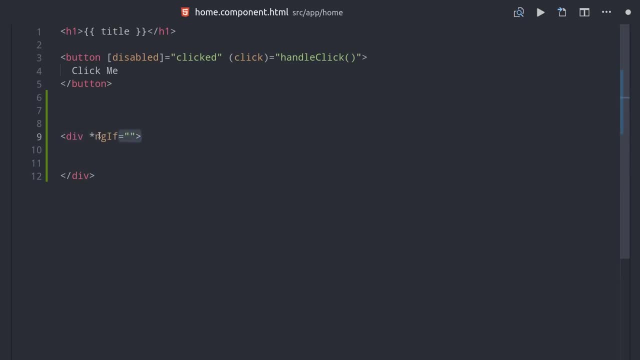 and any directive that starts with a star means it's a structural directive and controls how elements are rendered in the DOM. In this case, we're attaching ng-if to a div and it will only render this div if the right hand side resolves to true. 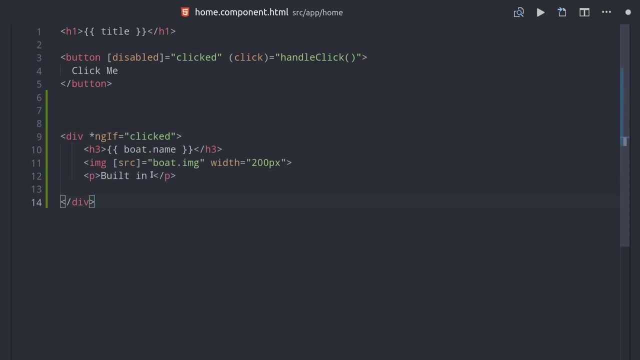 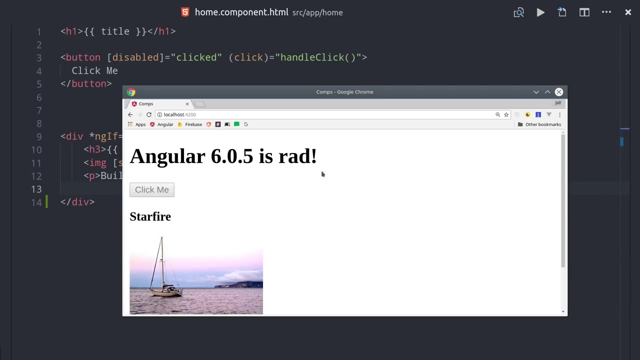 So, going back to our clicked property, we're only going to show this boat data if the button has been clicked. When we open the app, you can see that it looks just like it did before, but when we click the button, it displays our boat data. You'll end up using ng-if. 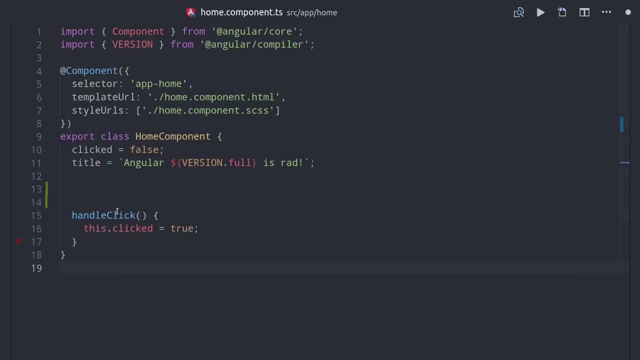 all the time in Angular, and there's one other directive that you'll use very frequently as well, which is ng-for. You can use it to loop over an array of data. So let's imagine we have an array with multiple boats in it. We've already mapped out how we want each boat to be displayed, but instead of using 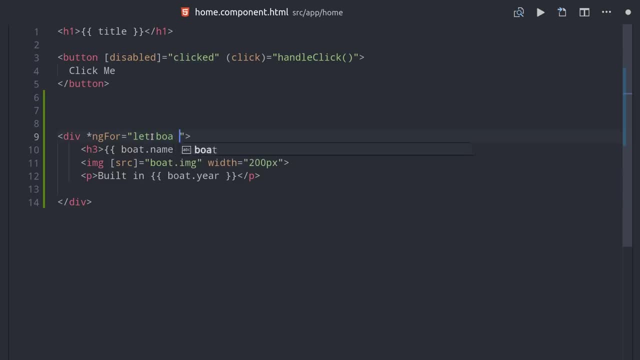 ng-if. here we can replace it with ng-for. Then we'll iterate over the boats array by saying let boat of boats. Then the div that this directive is attached to will be rendered for each item in that array. If we open the app, you can see we now have multiple boats utilizing the same. 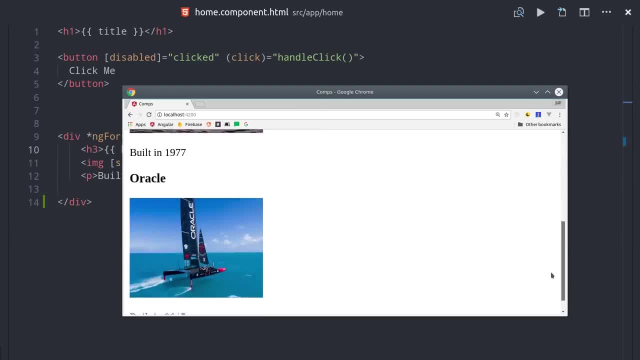 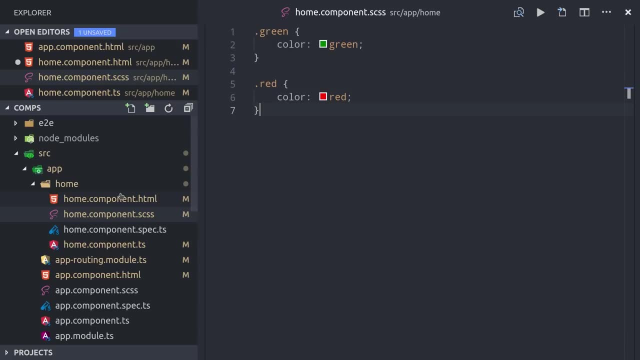 presentation logic. So those are super powerful. but another thing you often want to do is display different CSS classes conditionally based on some logic in your type script. Just as a basic example, let's imagine we have a green and red CSS class. 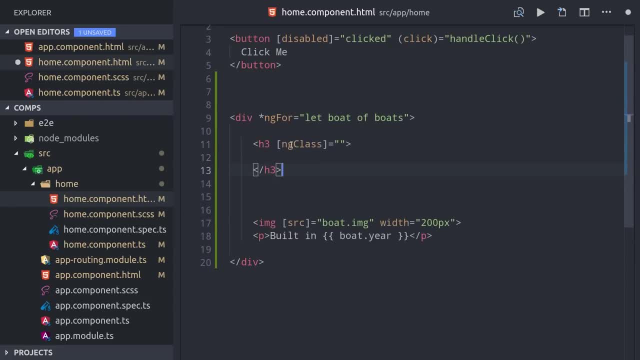 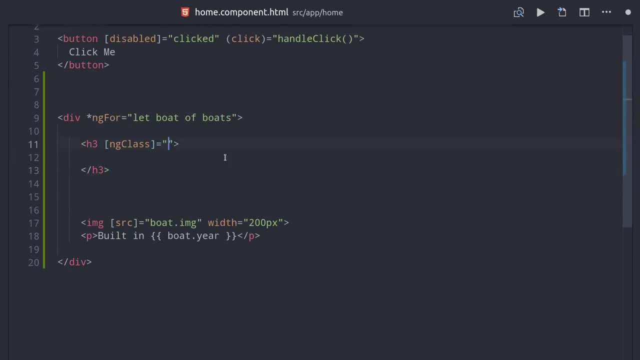 We can use the ng-class directive to control which CSS class gets applied to the h1 tile based on the name of the boat. So we'll pass the directive in object where the left-hand side of each object property is the CSS class we want to apply, then the value, or the right side is an expression. 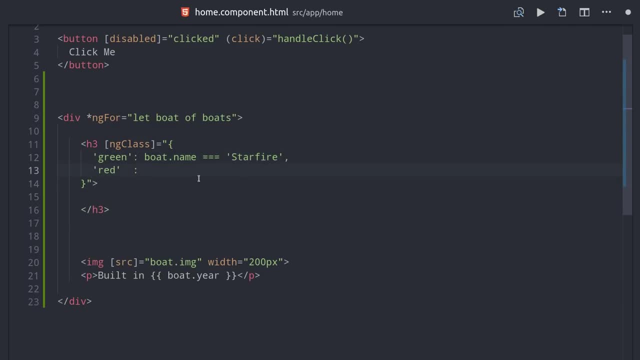 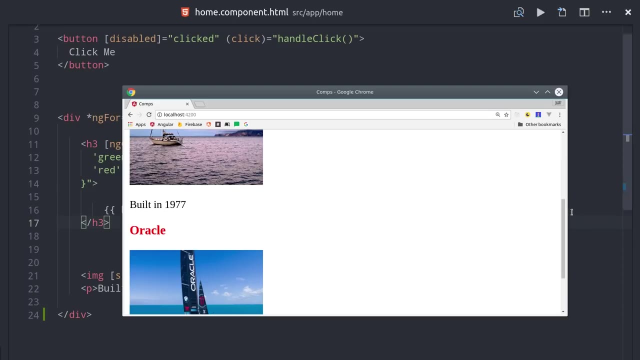 that resolves to true or false, which in this case will either be: boat name equals Starfire or boat name equals Oracle. Now we get a different color for each title based on this logic. So far we've only looked at built-in directives in Angular, but you can also build your own custom directives. Let's go ahead and. 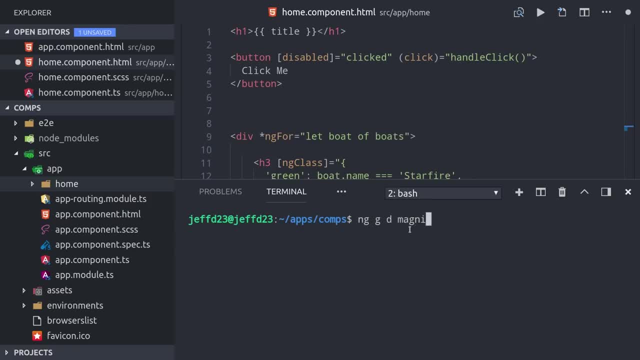 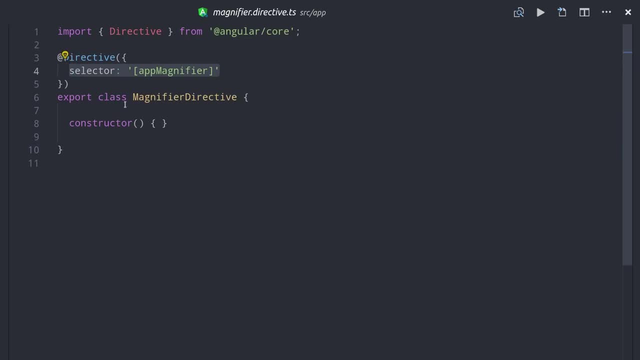 build our own with the Angular CLI by running an ng generate directive, which we'll call magnifier. that will increase the size of an image when it's hovered over. Overall. this looks pretty similar to a component, but the key difference is that there is no HTML template or CSS styles. Instead, it's used as an attribute. 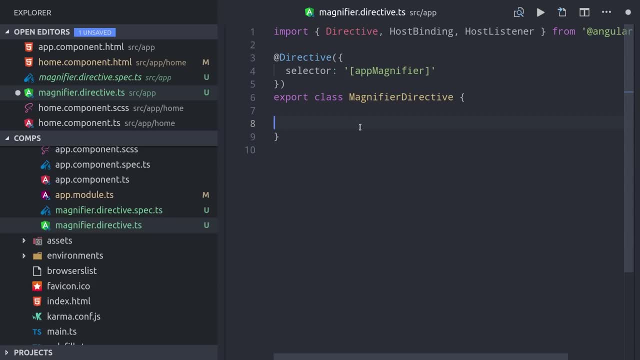 on an HTML element. This particular directive will be used to modify the width of an image element so we can bind to the host elements width by using the host binding decorator. Then any image that uses this directive will start with a width of 200.. Then we also want to listen to the mouse enter event to know. 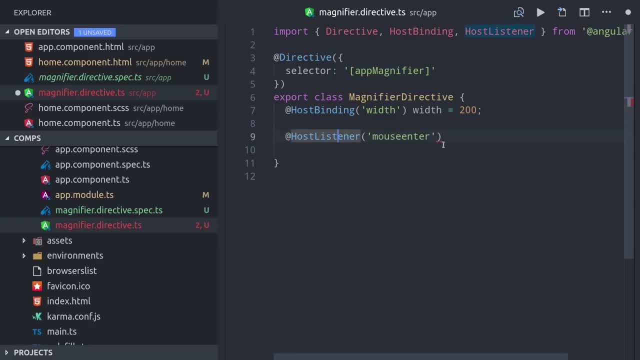 when the user is hovered over the image with their mouse. With that, we can use the host listener decorator, pass in the DOM event that we want to listen to and then define a function to handle this event. In this case, what we want to do is really simple. 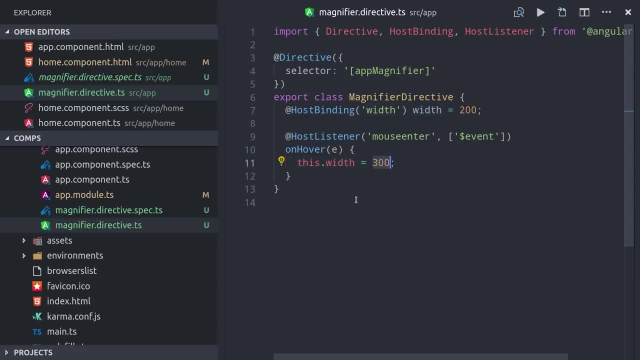 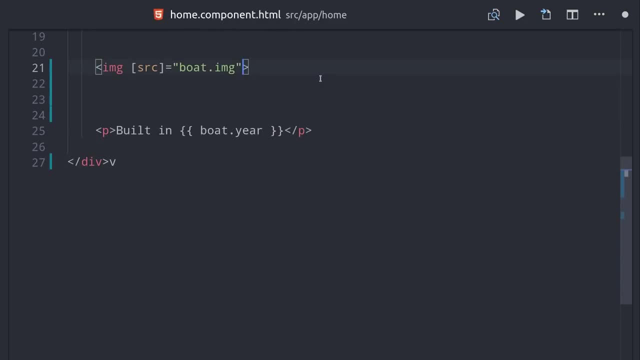 just increase the width from 200 to 300.. Now we'll switch back to the HTML in our component and we currently have an image in there that displays the boat image with a width of 200.. Let's go ahead and take this out and replace it with the app magnifier directive. 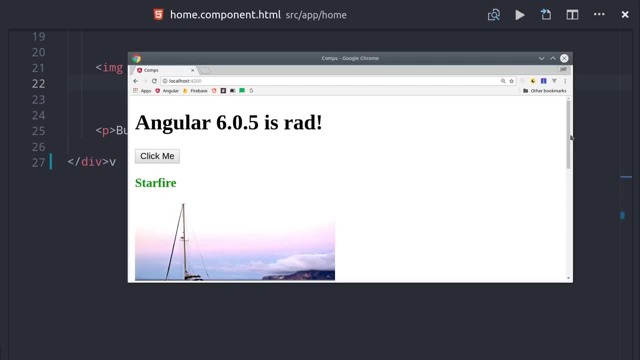 If we go back to our app and hover over the images, you'll see that they're resized as soon as we hover over them. Not the most useful thing in the world, but you get the idea of how you can use components and directives together to write really dry, reusable code. There's another mechanism in. 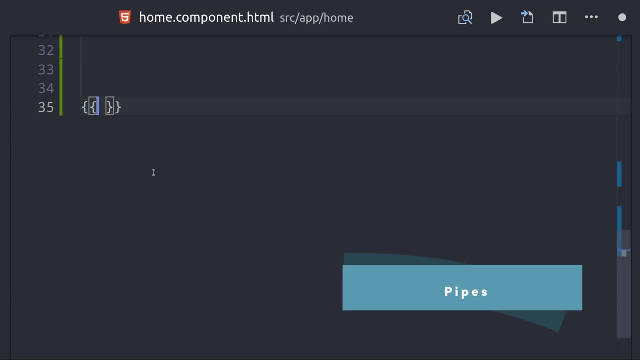 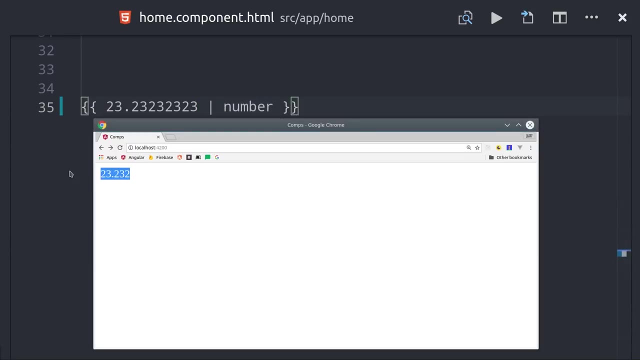 Angular that helps us write reusable code called pipes. A pipe is always used in an interpolated value in the HTML, So let's imagine we have a big number here. we can use the built-in number pipe to round this down to three decimals. Angular has some useful built-in pipes, but the real power. 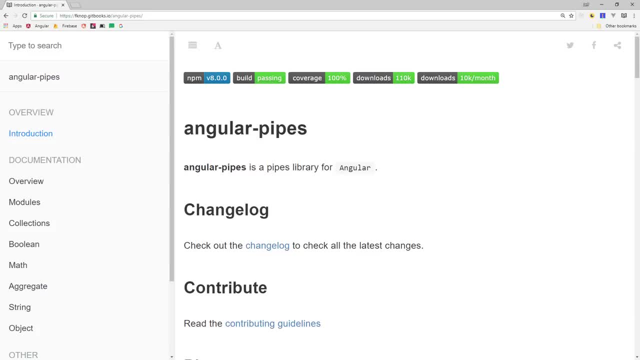 comes when you start building your own custom pipes And chances are somebody's already written the code that you need for your use case. so make sure to check out the Angular pipes guide if you want to learn more about that. So let's go ahead and take a look at some of the 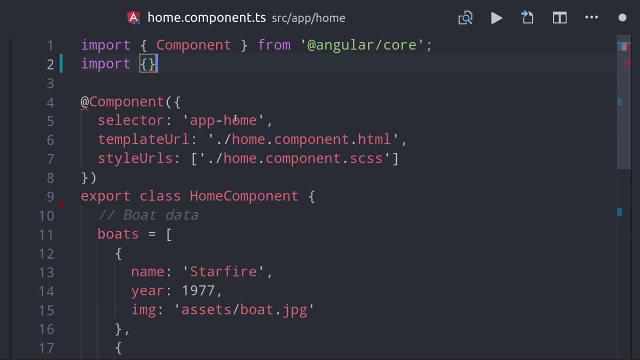 GitHub repo for a full list of examples. There's one really special pipe that I want to talk about now, which is the async pipe. In a web application, you're commonly fetching data asynchronously as a promise or an observable, and the async pipe allows you to do this automatically in a predictable. 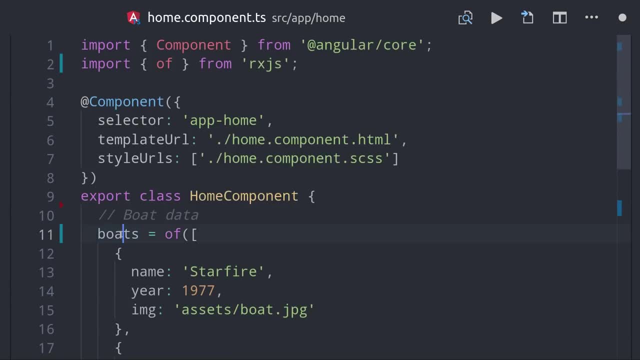 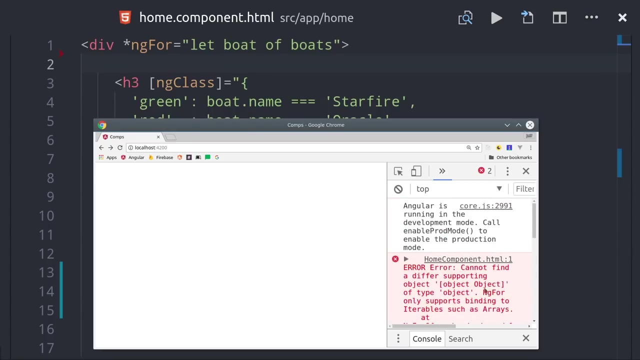 way, directly in the HTML. In this example I'm converting our boats array into an observable by using the rxjs of method, So now it becomes an observable object. so our regular ng4 loop isn't going to work. What we can do is simply add the async pipe to our for loop and now it's going to convert that. 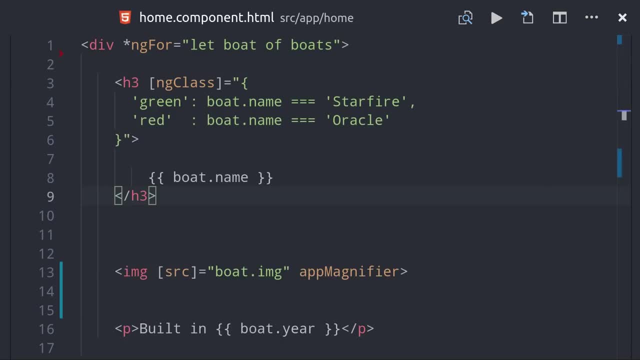 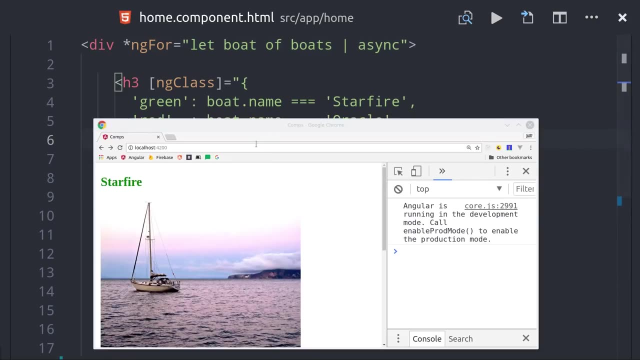 observable to an array by subscribing to it and in addition, it also unsubscribes when this component is destroyed. That's a whole other subject on rxjs, but just know that it's a very useful mechanism for simplifying your Angular code. In a real app, we'd probably be fetching these. 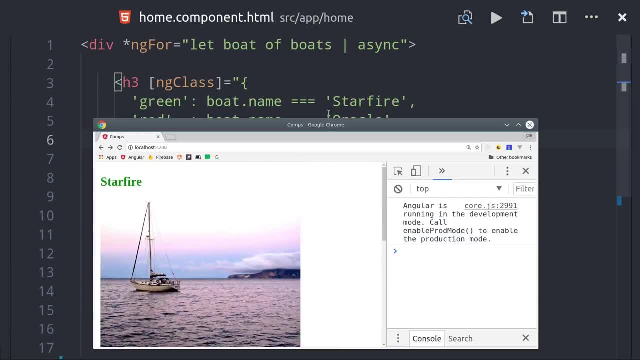 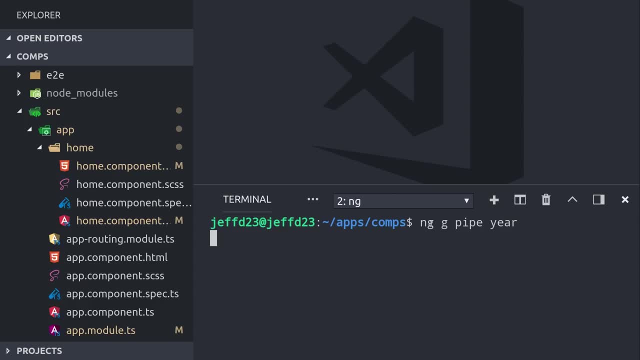 boats asynchronously from a database, and the async pipe allows us to treat them more like asynchronous, plain javascript array. At its core, a pipe is very simple. it's just a function that takes in a value and then spits out another value. Each of our boats has a year property on it. 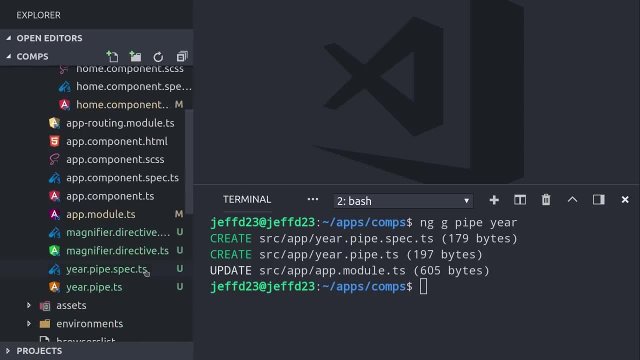 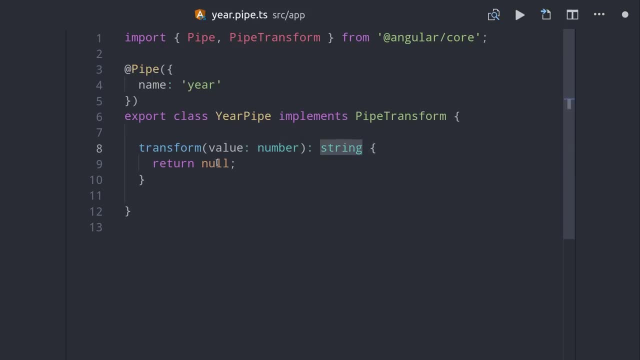 Let's say we want to only display the last two digits in that four digit year. All we have to do is go into our custom pipe and then implement this transform method. The value represents whatever value is inside the handlebar syntax in your HTML. 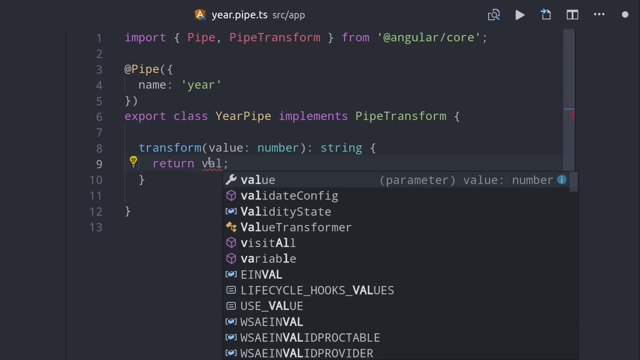 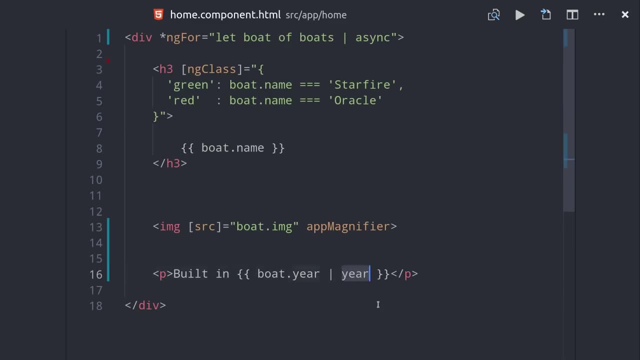 Then the value you return is what you want to be shown in the HTML. In this case we'll convert the number to a string and then grab the last two elements on that string. Then we can go add it to year in our HTML and then if we reopen the app, we'll see that we only get the last two numbers. 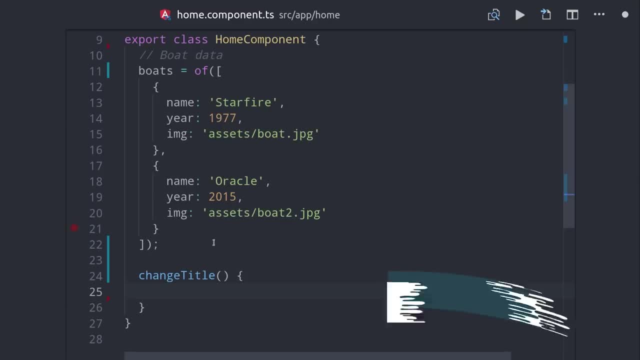 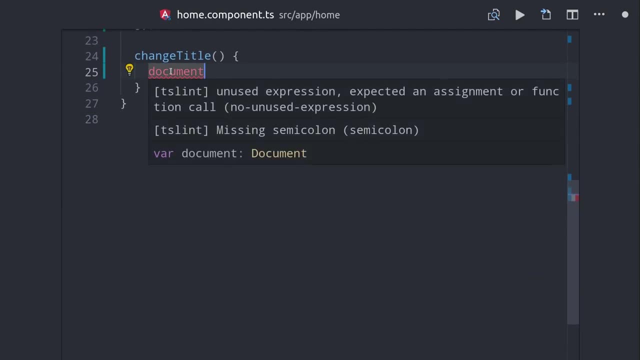 on the year. So now that you know a lot about components, pipes and directives, I want to talk about a concept that's really important for Angular developers and that's never touch the dom. If you're an experienced javascript developer, you're probably used to doing something like this. 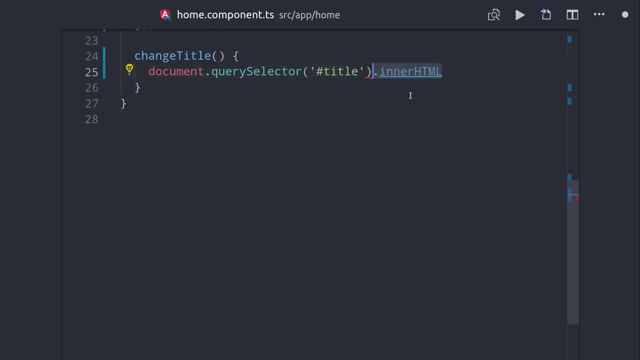 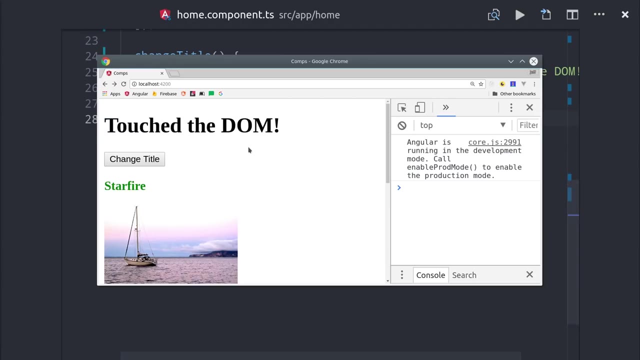 where you call document query selector, then grab some element in the dom and change its inner HTML. and when you're building a progressive web app, this code will work perfectly fine because the dom exists in a web app. So let me talk about that. So when you're building a progressive web app, this code will work perfectly fine because the dom exists in a web app. 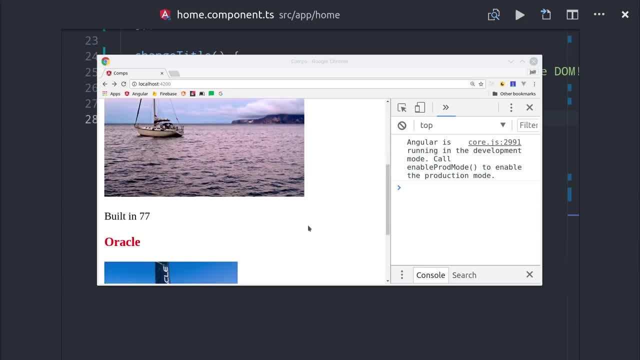 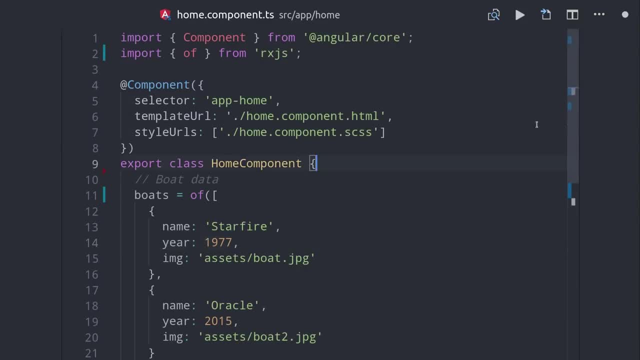 app. But if you write code like this and you ever want to do server-side rendering or build a native mobile app, this code will not work because the DOM does not exist on other platforms. So now you know why the use of libraries like jQuery are generally discouraged in Angular. Now let's switch. 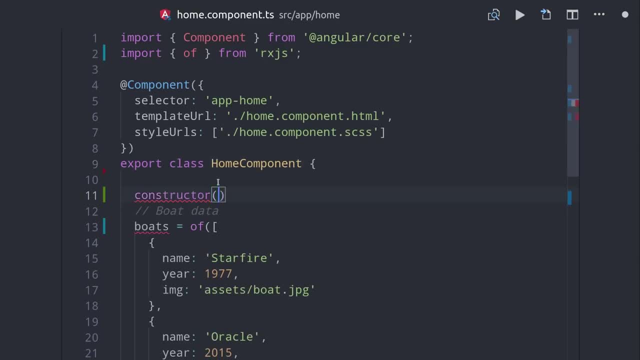 gears into the component lifecycle. A component is just a class, so the very first thing to happen in its lifecycle is the constructor is fired. But components have relationships with other components and they have bindings that are initialized in the HTML. so things get a little. 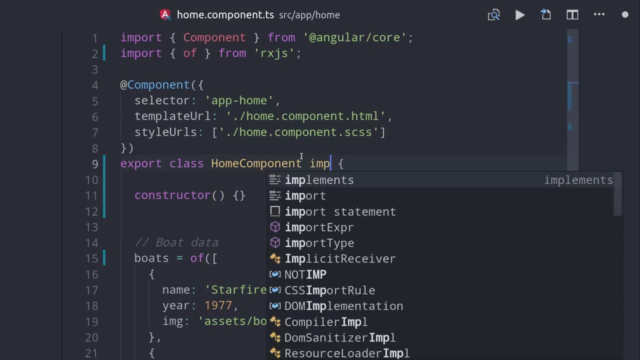 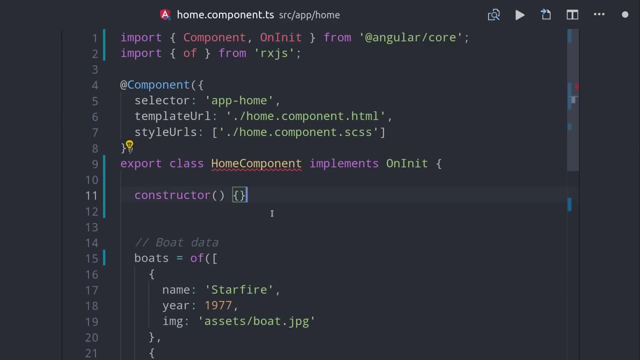 bit more complex. In Angular. you typically don't do anything in the constructor except add your dependencies, And that's because your property bindings aren't guaranteed to be available until you run ngOnInit, which is the first time change detection runs in this component. So the 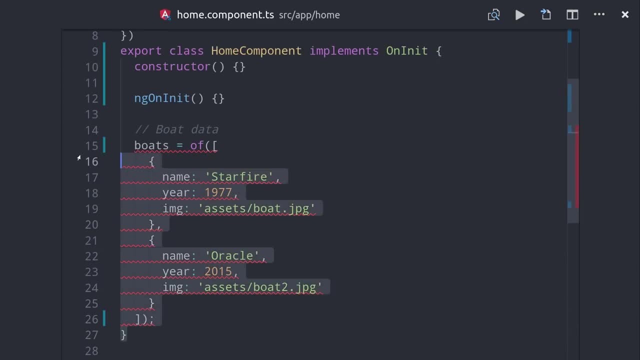 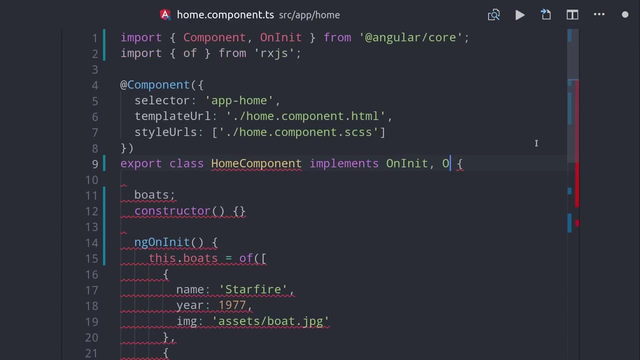 onInit lifecycle hook is where you do all of your setup. Maybe you're fetching data from an API or you're setting up a reactive form or something along those lines. I'll go ahead and add our boats observable. The last thing to happen to a component is that it's destroyed, which triggers the onDestroy. 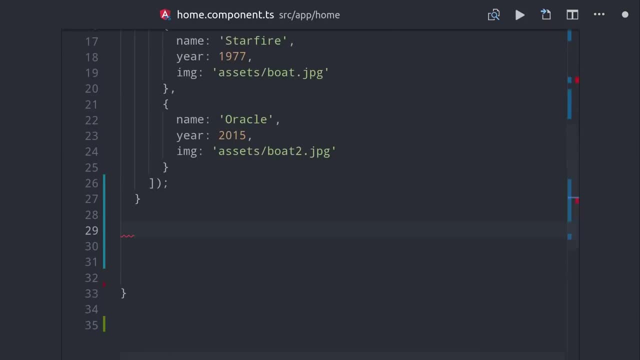 lifecycle hook. This is where you would do any teardown for your component In Angular that is commonly unsubscribing from an observable, to prevent things like memory leaks and performance issues. onInit is by far the most common hook that you'll use, but if you have child views inside of 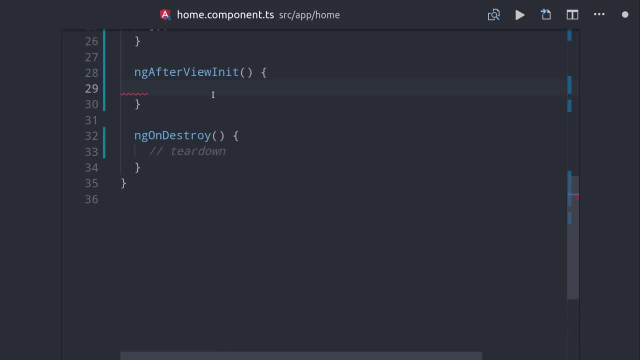 your component. you might also want to use afterViewInit, which will ensure that your child views are loaded as well. Now that segues into a really important concept in Angular, which is change detection Behind the scenes. Angular is using something called zonejs that will listen for any events or asynchronous. 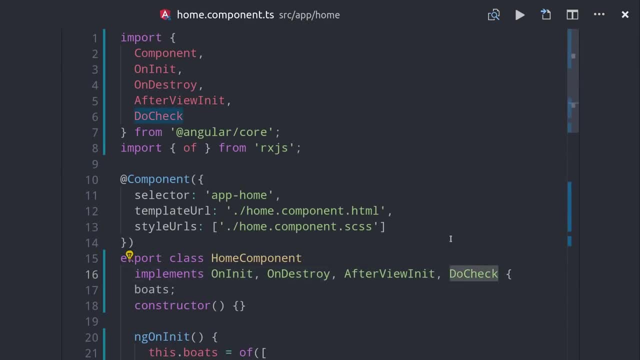 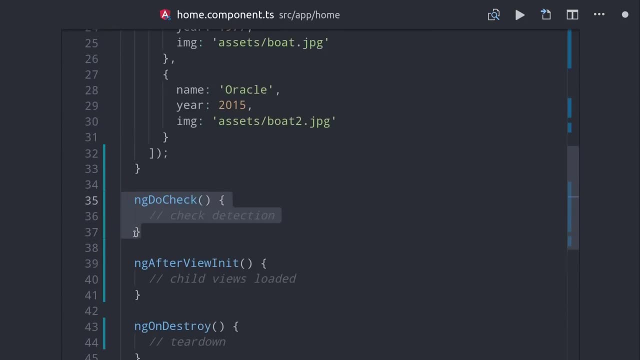 activity in your app and then rerender components as needed. You can determine when change detection is happening by using this doCheck lifecycle hook. You wouldn't normally use this to do anything significant, but it is useful for debugging at times If you're building an interactive app.